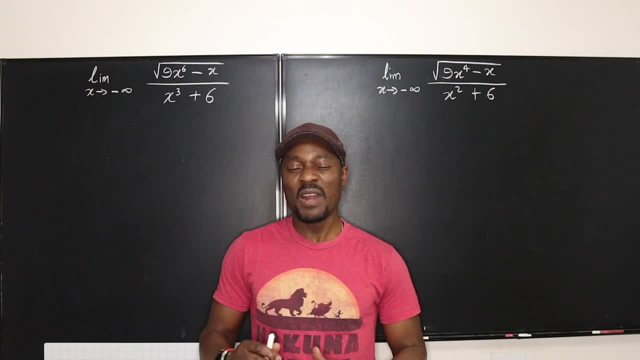 Hello, welcome to another video. If you were ever confused at any time about questions like this, when negative infinity puts you in trouble, where you don't know when your answer is going to be positive or negative, this is the video you need. Watch this video to the end Now. for some of you, 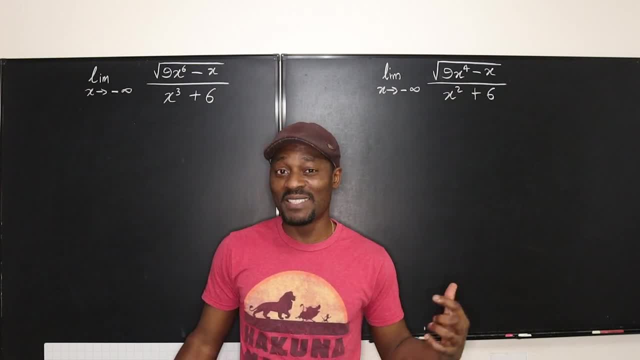 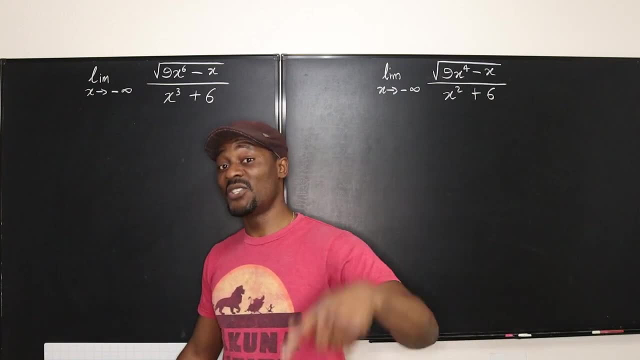 you don't need to watch it to the end. As soon as you understand the concept and why they are different, you just go ahead and stop watching. But make sure, before you leave, give this video a like, share it, tell your friends about it, because this is going to help a ton of people. 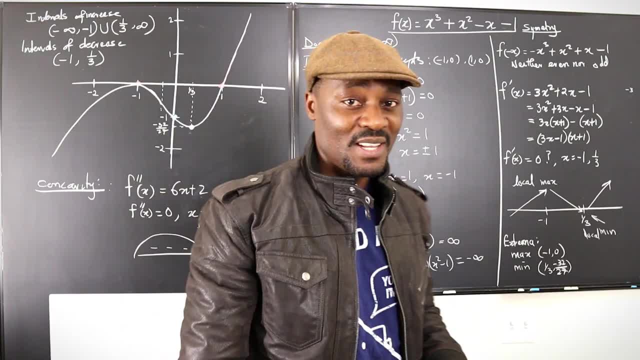 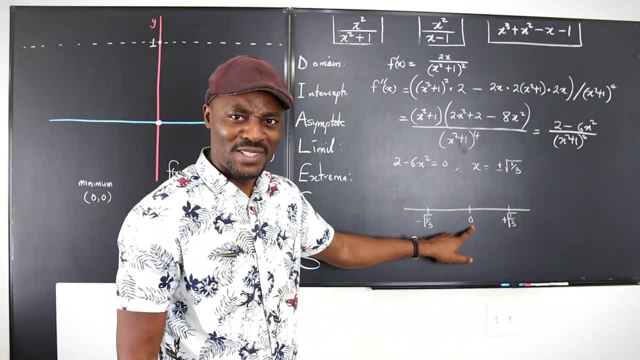 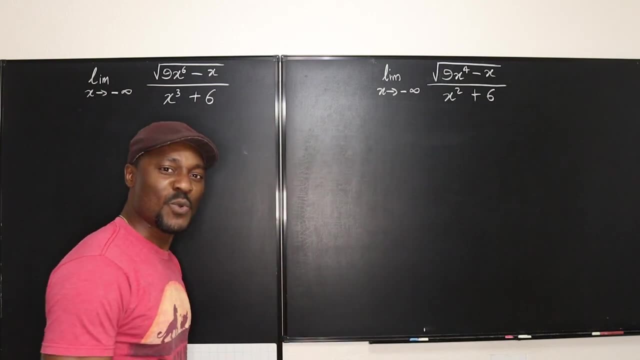 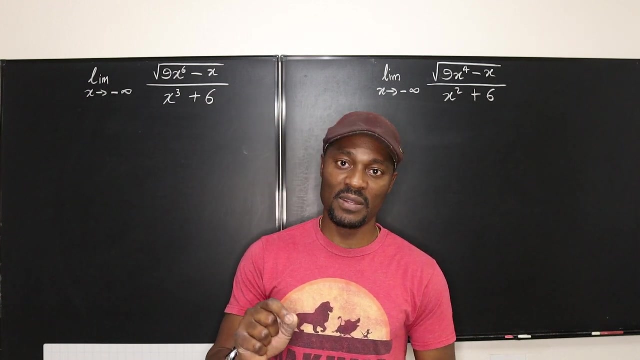 Let's get into the video In order to understand this concept. the first thing we have to talk about is this thing called the square root of x squared. It's a concept that keeps popping up, and you just have to understand what happens when you take the square root of x squared. Now look at this. I can tell you. 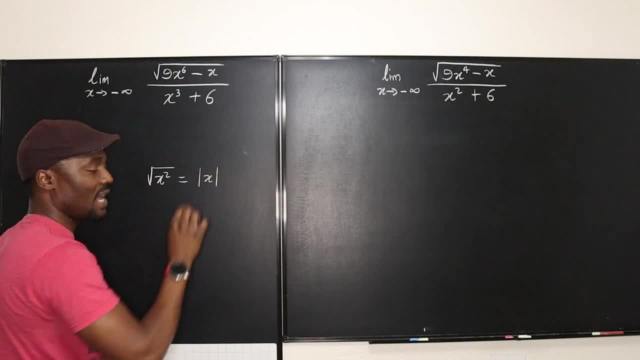 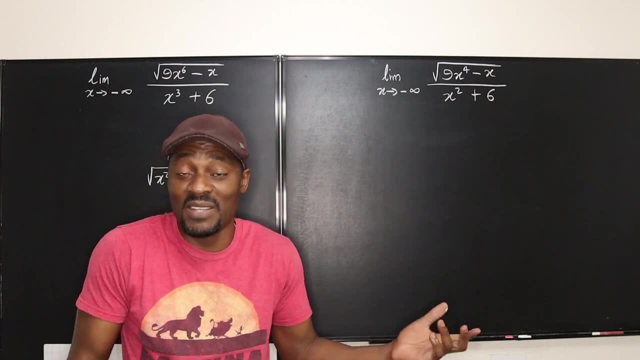 that the square root of x squared is always the absolute value of x, Which means, when you take the square root of x squared, your answer is either positive x or negative x, depending on whether x is positive or negative. Yeah, it's as simple as that, Because 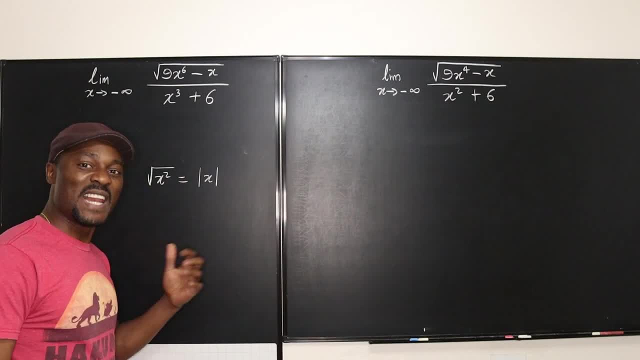 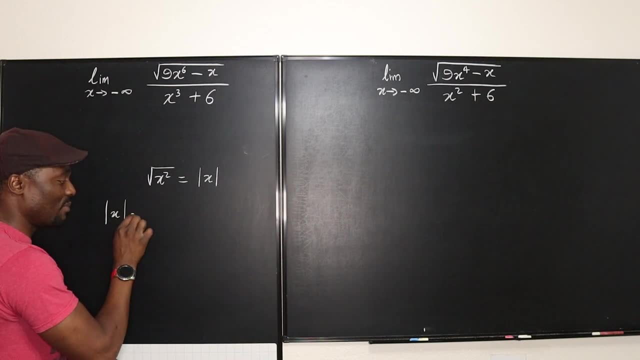 it's possible that the square root of x squared is x, or the square root of x squared is negative x, And that's why we say the square root of x squared is the absolute value of x, which you write this way: the absolute value of x, remember, is equal to x. Okay, If x is greater than zero, Or it is. 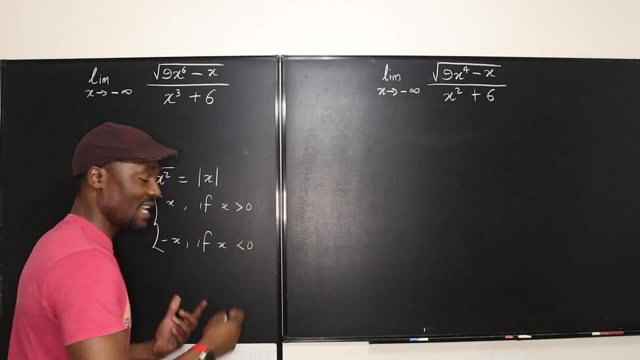 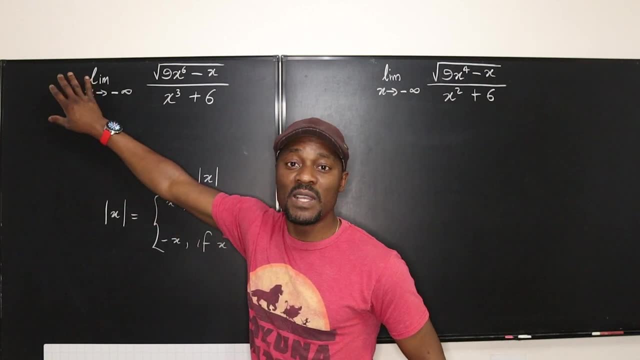 equal to negative x. If x is less than zero, that is, x is negative. You have to have this concept on your mind. Okay now, how is this relevant? The question tells us that what we're dealing with, x, is going to negative infinity. Therefore, it is not possible for x to be positive by the 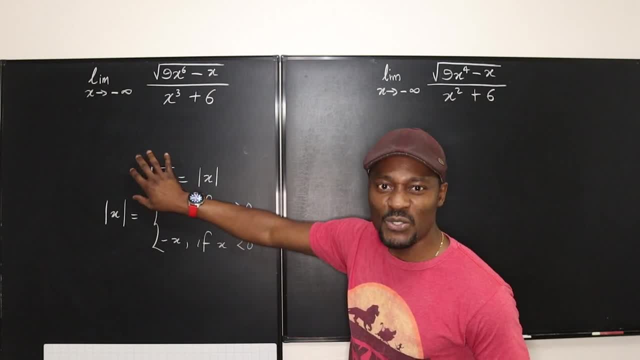 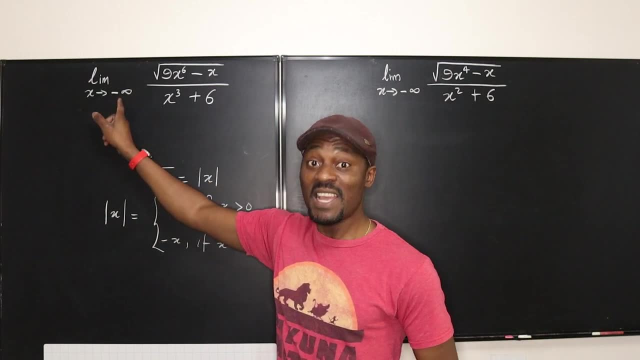 time we do what we're supposed to do. So when you take the square root of x squared, your answer definitely has to be a negative number. It cannot be the positive because x is approaching negative infinity, That's, it's a very, very negative number. Remember that. 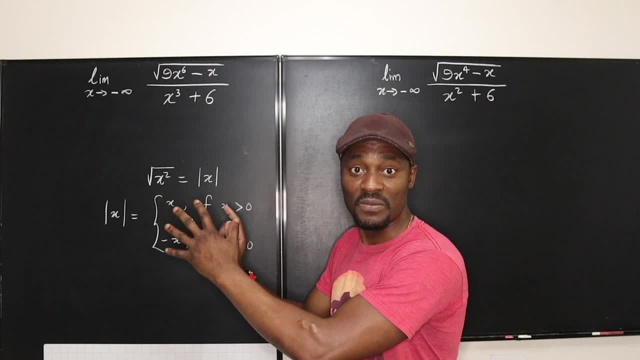 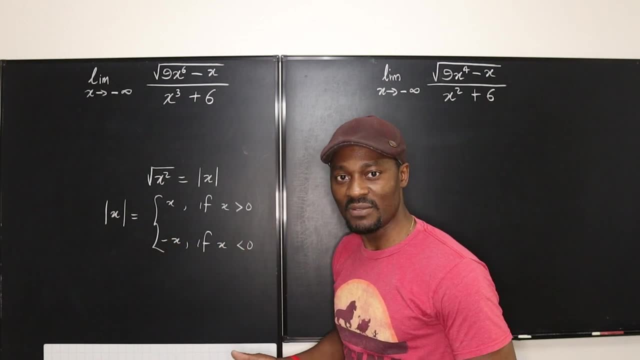 So when we take the square root of any x squared in the problem we're solving, we're going to be getting the negative option, not the positive option. Get this concept and then I'll take you back into the course, into the question. Okay, So now that you understand that the square root of x 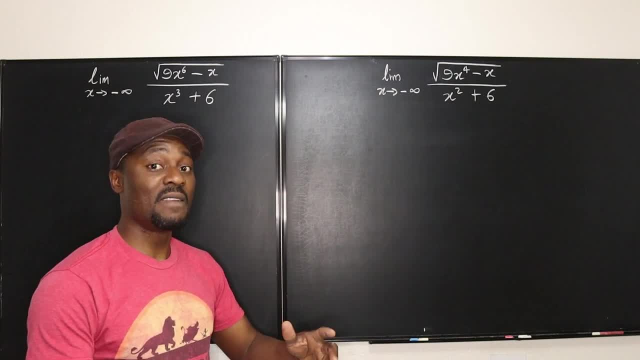 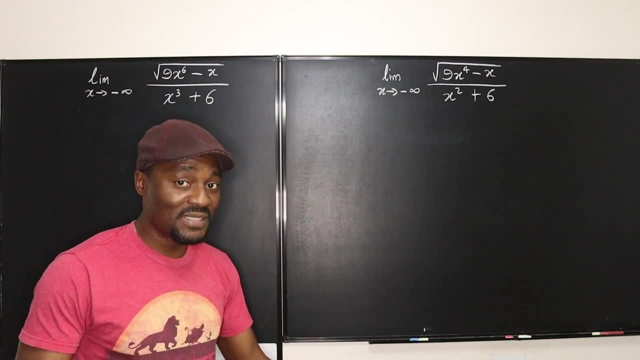 squared is the absolute value of x, which gives us two options: positive or negative. but with the weirdness of this problem, they tell us that x- you can see, in both cases x is going to a negative infinity. That simply means that the option you would pick will be the negative option. 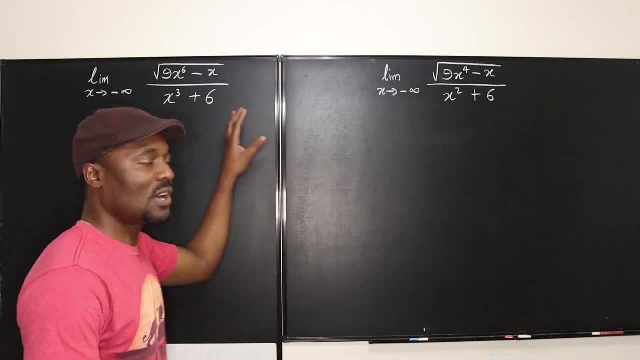 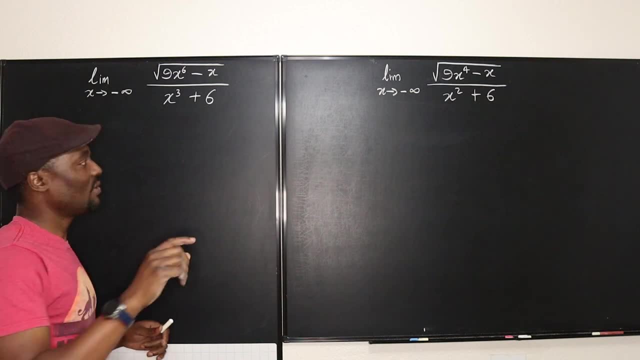 But how do you use it in this problem? How do you use it here? How do you use it there? Now, let's start from the top Now. if you've solved this before, or you've seen my other video that addressed this question, you'll notice that the major thing you need to deal with all of these. 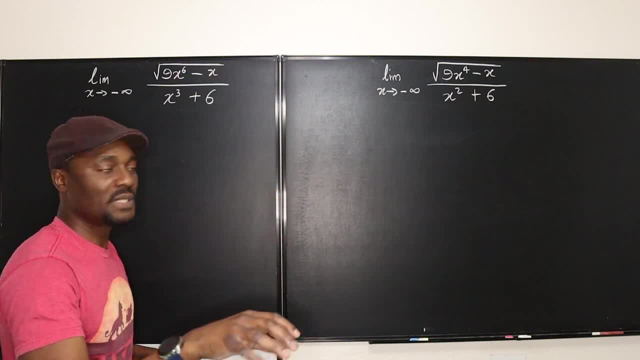 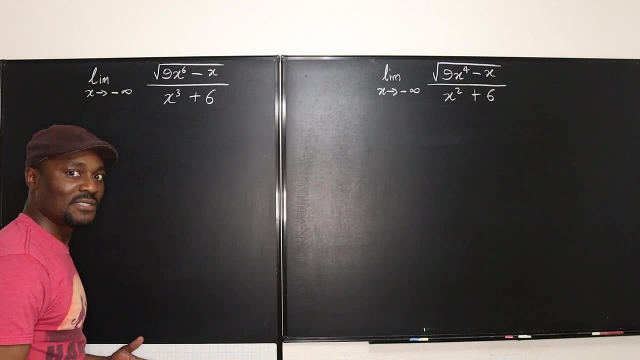 will disappear somehow. I'm going to show you how they'll disappear. Your major focus is on this term here that has the highest exponent under the square root side. So let me explain. If somebody walked up to you as a math, as a brilliant math student, and said what would be the square root? 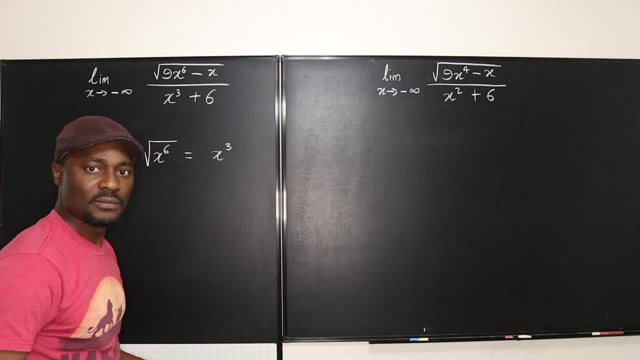 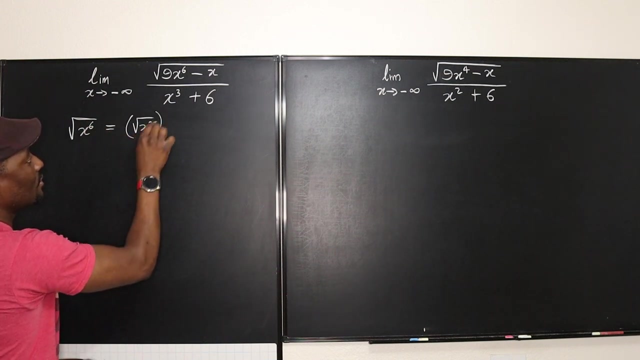 of x to the sixth, You'll straight away say it's going to be x cubed. Let me show you something. Do you know that, instead of you writing this, the square root of x to the sixth is the same thing as the square root of x squared to the third? You see, And we can rewrite. 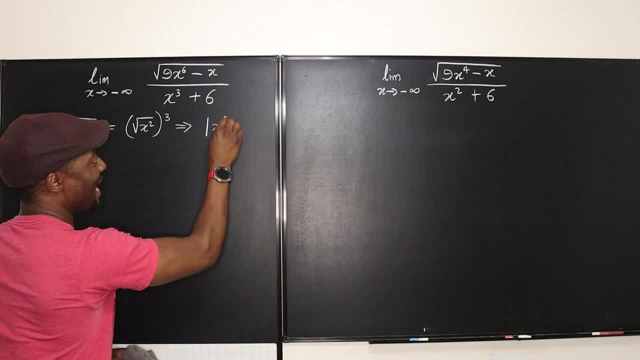 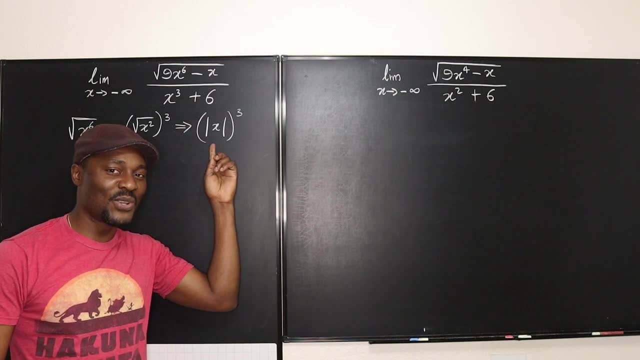 this expression to mean the absolute value of x raised to the third. Now, which option are you going to pick here? Are you going to pick the positive option or the negative option, The negative option? You're going to pick the negative option because x is going to a negative. 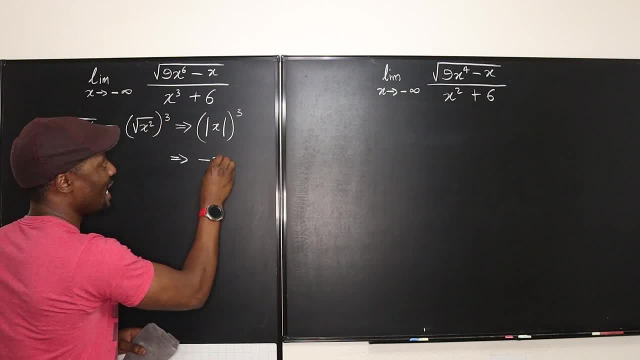 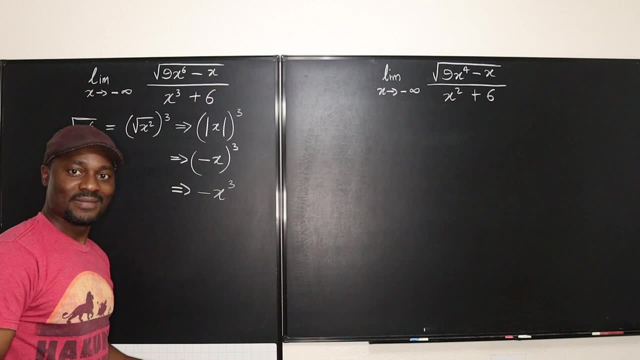 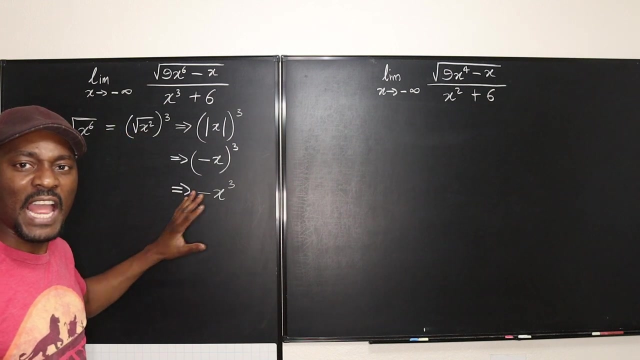 infinity. So the answer to this question is going to be negative x to the third. What is negative x to the third? It's negative x cubed. Now you understand. You understand why the negative sign stays. I want you to go over this again in your mind and know it, that that's why the negative 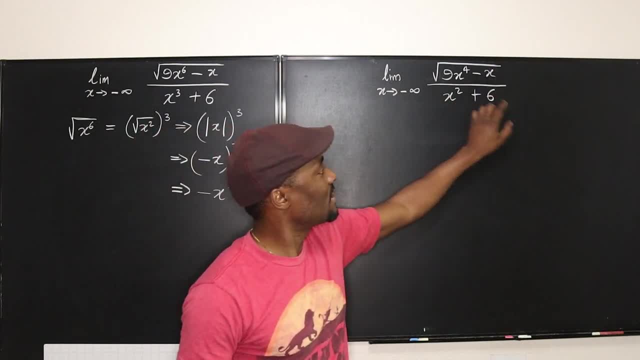 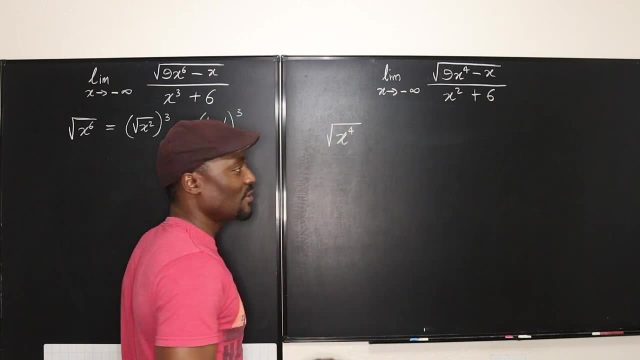 sign stays. Let's try that here. All of these will disappear, except for this one. That's what we need to deal with. So let's go And write the square root of x to the fourth, The square root of x to the fourth. Well, if somebody. 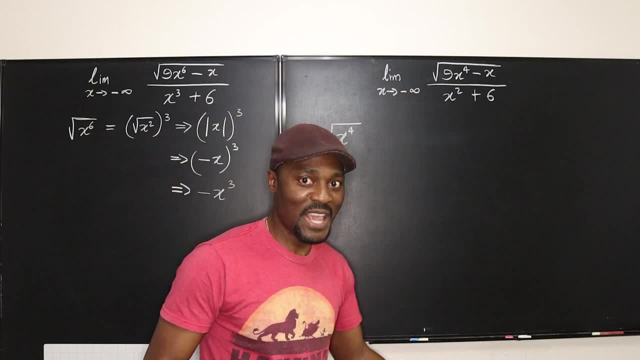 finds you on the street and says: what will this answer be? You'll say: it's going to be x squared, OK, but let's rewrite it because you don't know. it's going to be x squared, OK, we're going to. 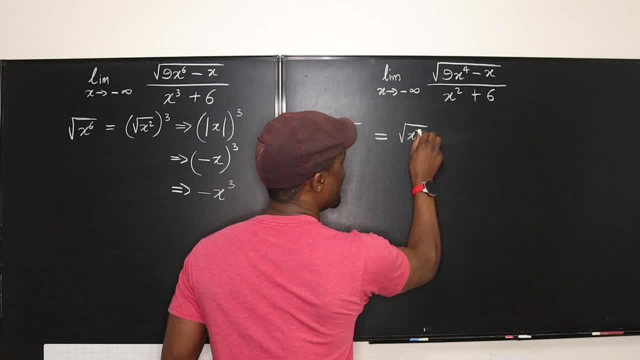 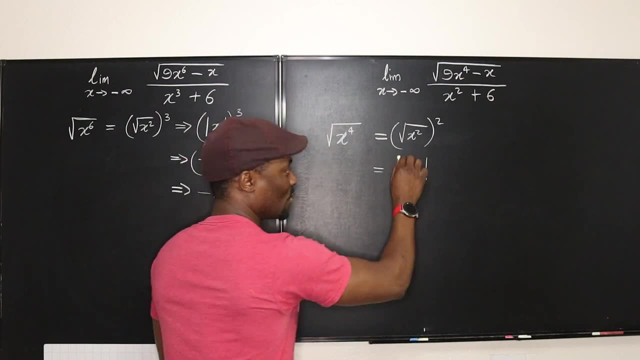 rewrite it just the same way we did this. It's going to be the square root of x, squared, then squared. What is the square root of x squared? It's the absolute value of x squared. OK, which option are we going to pick? Is it the positive or the negative? 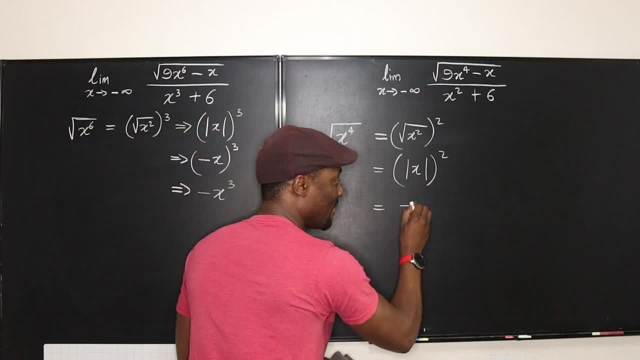 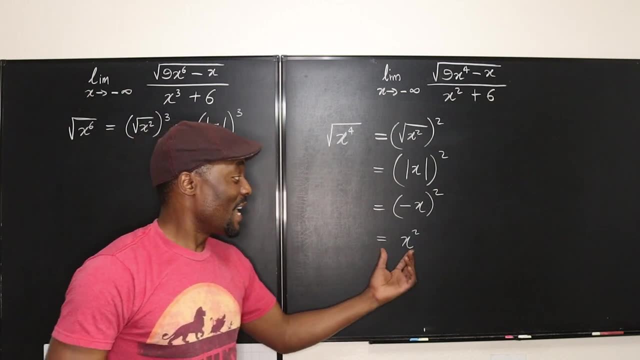 The question says x is approaching negative infinity. so we're going to pick the negative option, negative x, But then we're going to square it. If you square negative x, what do you get? You get x squared, So you notice that this is going to give you a positive. 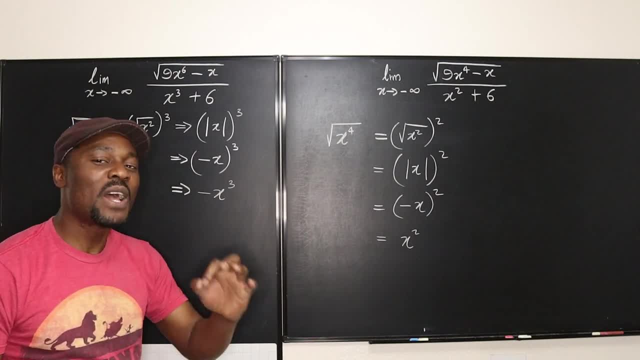 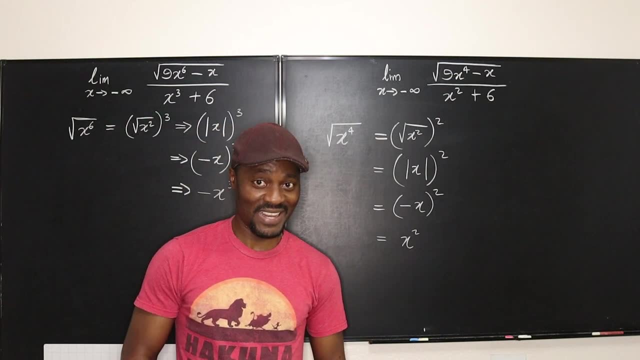 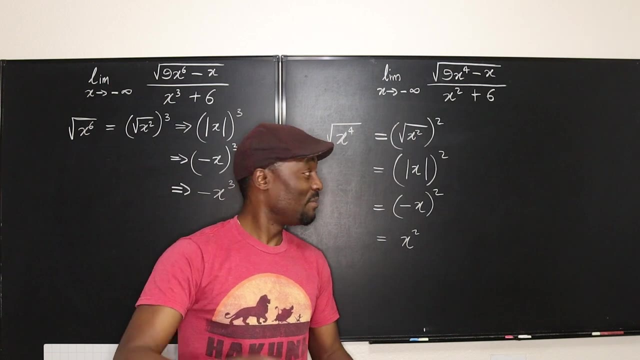 output. This is going to give you a negative output. That is what is responsible for the difference in the answers. Do you understand? Now, at this point, if you know what to do, give this video a like, share it, tell everyone about it and don't stop learning. But if 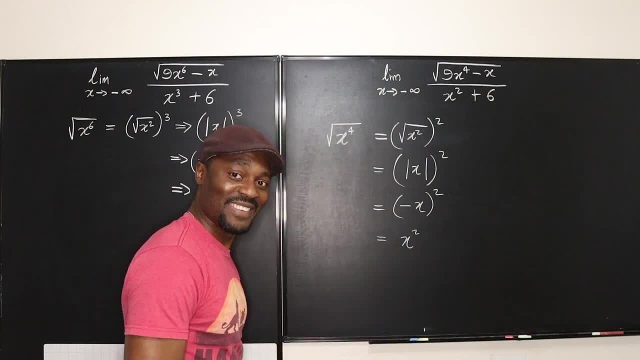 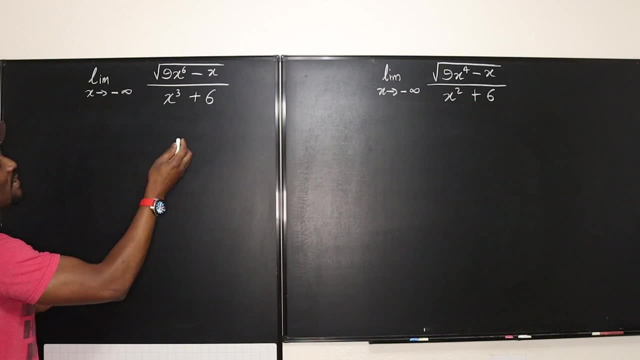 you don't want to do it with this information. you just got watch the rest of the video. Let's do it, OK. so I'm just going to solve this, with the understanding that you know what I'm going to do as I solve it. OK. so the first thing to do is to get rid of the 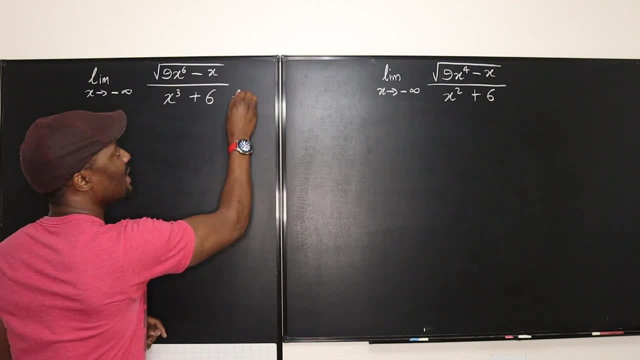 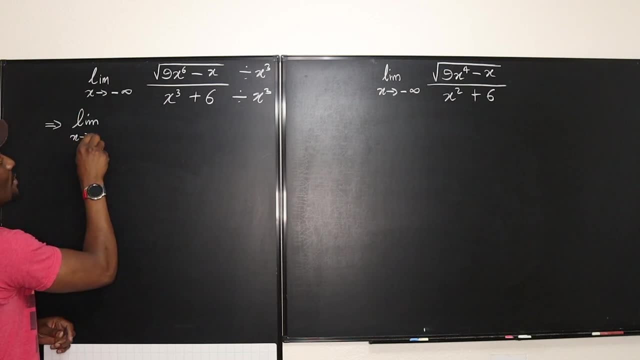 term with the highest exponent in the denominator, which is x cubed. So I'm going to divide this by x cubed, and I'm going to divide this also by x cubed. OK, so that tells us that the limit, as x goes to negative, infinity will be. let's take care of the top part, It's. 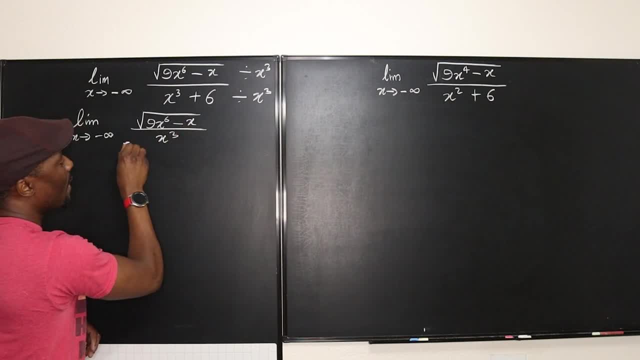 minus x divided by x cubed. OK, I'm just going to leave that, and this is going to be x cubed over x cubed, plus 6 over x cubed. Now, what do we get from here? This is going. 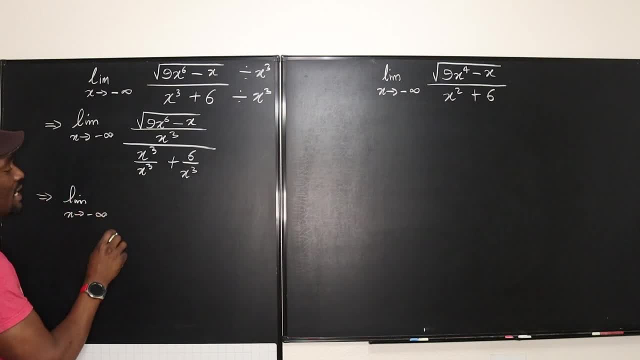 to give us the limit, as x goes to negative infinity. And now, when you're dividing a square root term, let me quickly explain that. So look at this: Instead of saying the square root of 9 divided by 3,, remember this is going to give you 3 over 3, and then you're. 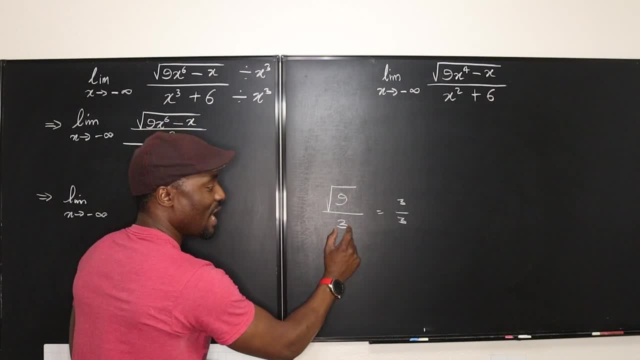 going to get 1.. But there's another way you could get this answer: Take this 3 and push it under the square root sign. But when you push it under the square root sign, you are going to square it so that it looks like this: It's a square root of 9.. Instead of 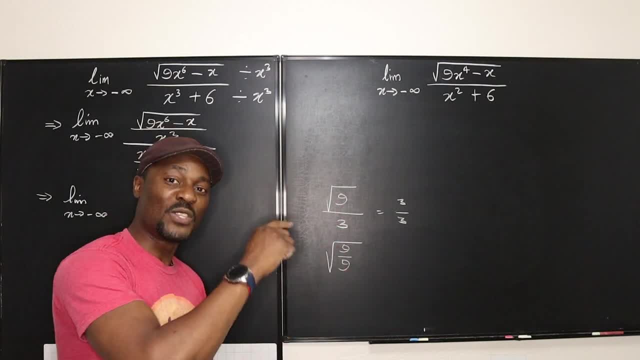 9 over 3, it's now going to be 9 over 9.. You have to square this so that when you take the square root of it again, it will come back out as just 3.. But if you push it under, 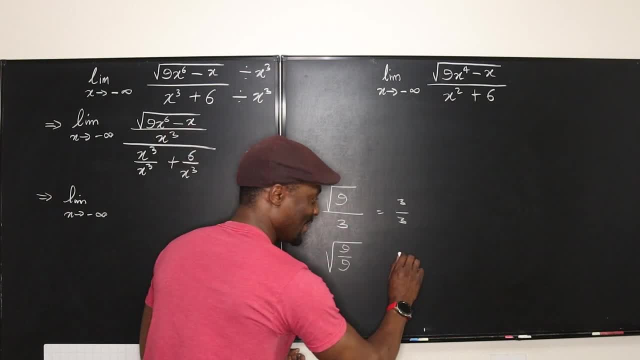 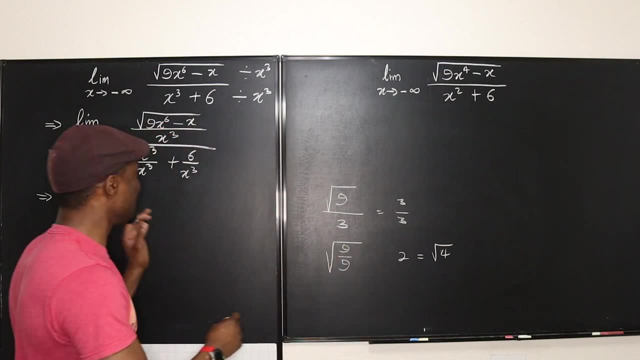 the square root sign, it becomes 9.. OK, the same thing. Instead of you writing 2, you can just write the square root of 4.. So when you push the 2 under the square root sign, you square the 2, and then it becomes 4.. So that's the idea that I'm going to employ. 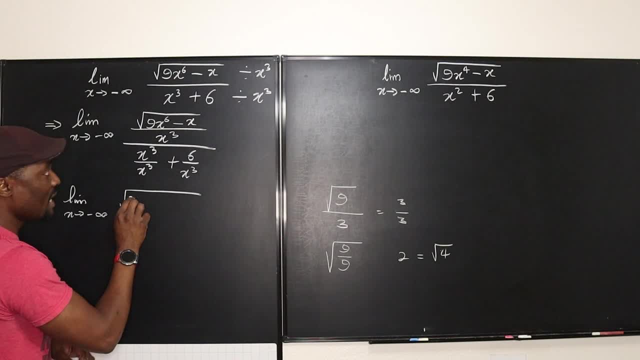 here. So I'm going to write this as the square root of 2.. 9x to the 6th. OK, over x to the 6th. See, I have squared this. x cubed, Now x to the. 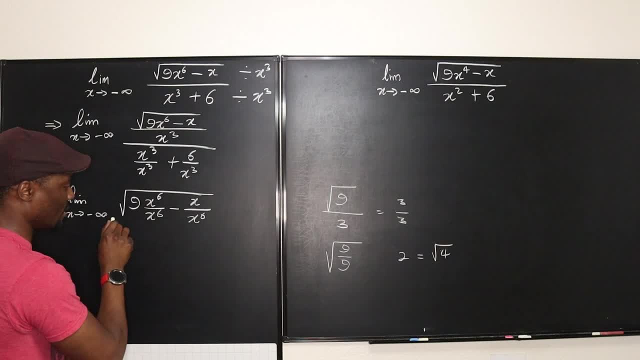 6th minus x over x to the 6th, Now both under the square root sign divided by. this is going to give me 1 plus 6 over x cubed. Now let's simplify. OK, now this is going to. 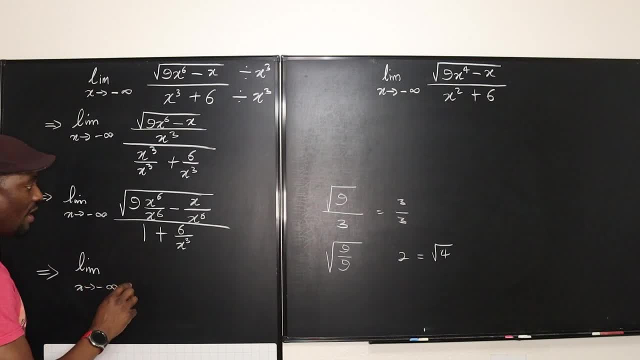 be the limit, as x goes to the negative infinity of Now. you see, what I have done here is that, as I divide, when I take this square root, let's just do it this way, Because I know my answer is going to be negative. it's always. 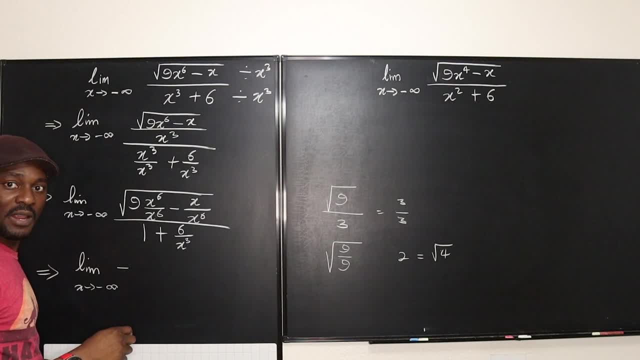 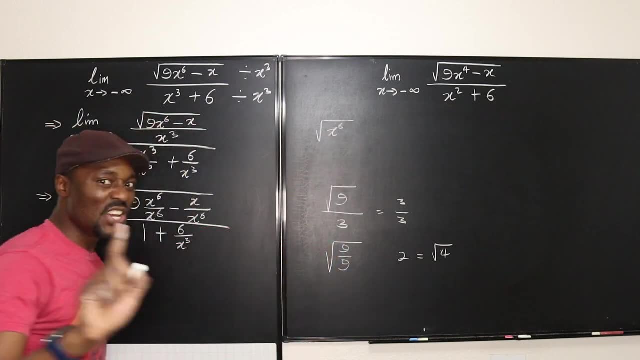 safe for you to put a negative sign here as soon as this x is going to disappear, because your answer is supposed to be negative. Remember that when you took the square root of x to the 6th, it did not really give you x cubed. Remember we didn't get x cubed, We got negative. 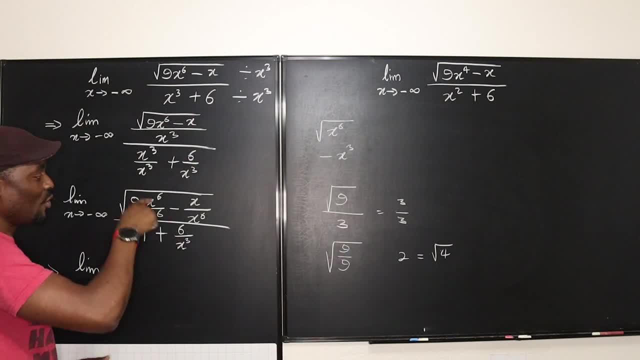 x cubed. So by the time you push this one in, OK, you're going to be getting negative, And because there's no room to write that negative here, it's better to write it outside the square root sign. OK, I think I would write it here. 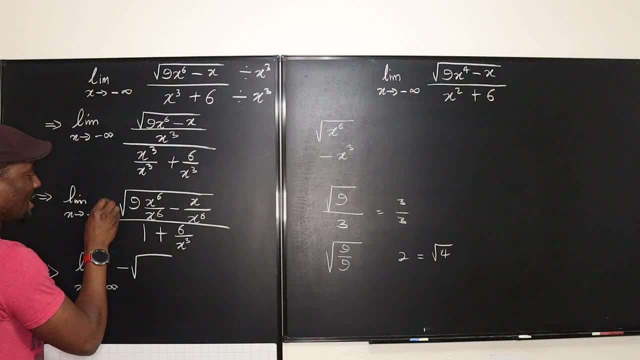 Better to put it in red so you recognize it. So it's going to be negative, OK, and from then on you can get rid of this. That's going to be square root of 9.. And this would be minus 1 over x to the 5th, divided by 1 plus 6 over x, cubed. Now we can evaluate. 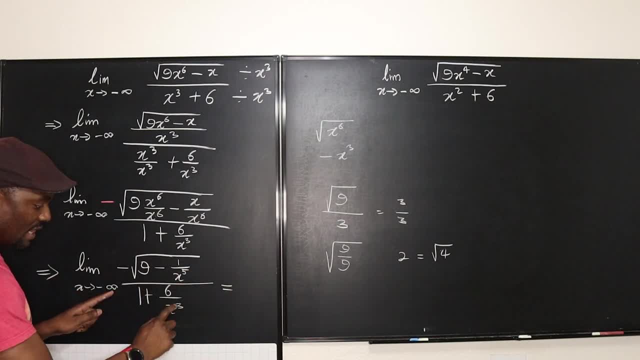 this: As x goes to negative infinity, this will become 0.. This will become 0.. You end up with negative square root of 9, which is going to be negative 3.. So that is the limit of this expression. There's another video I did previously. You can go. I think I did. 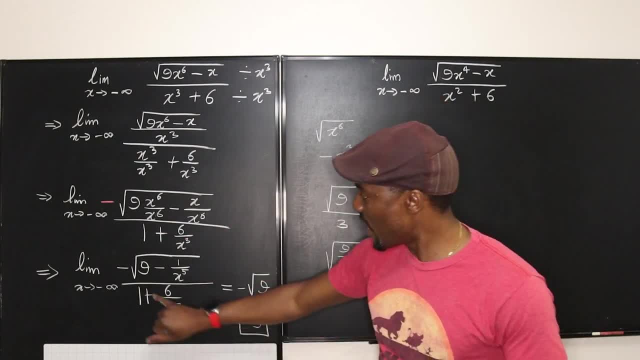 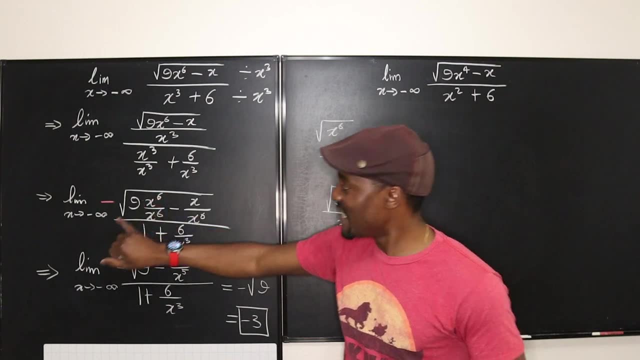 a lot more talking about that, But it's the same concept that I just explained. So you see why the negative shows up here From that original explanation that I gave that by the time you take the square root of x to the 6th, as x goes to negative infinity, your. 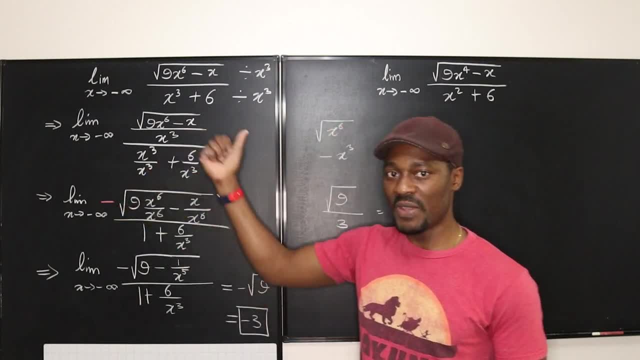 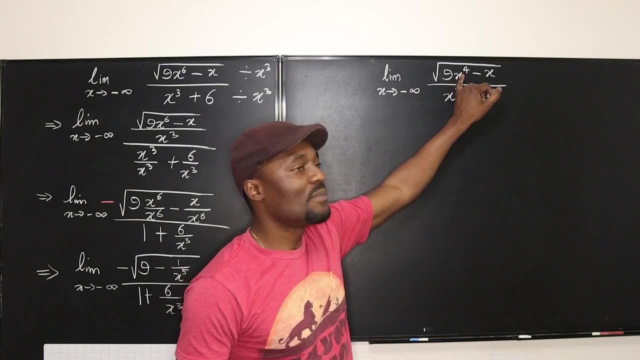 option will not be x cubed, It's going to be negative x cubed, based on that previous explanation. Now let's see what's going to happen on this side. So, as you see, because this is The square root of a square, by the time you square the negative it will end up being 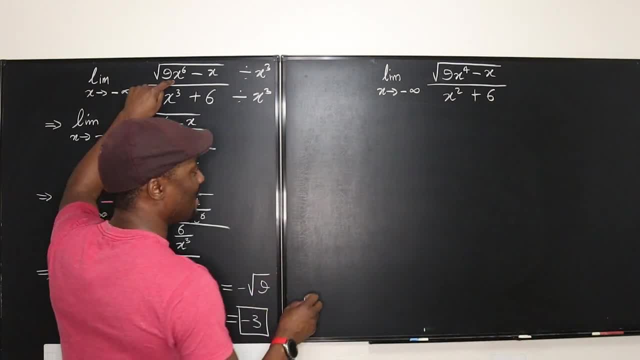 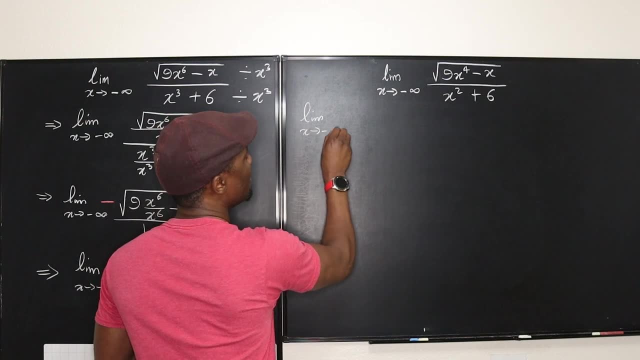 positive again. So you see the difference, Remember. so now you see that Let me just finish this. So let's just get into this one. It's the same thing I'm going to do. The limit as x goes to negative infinity. well, I'm going to divide this by the highest exponent. 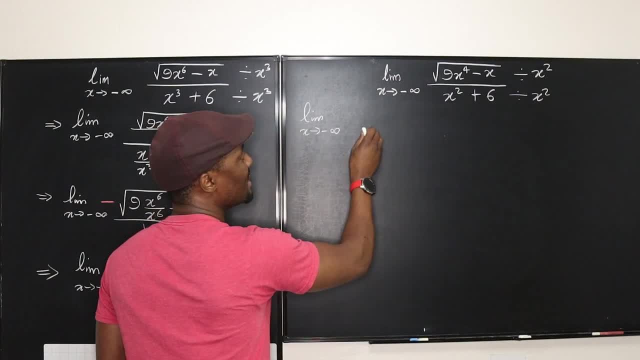 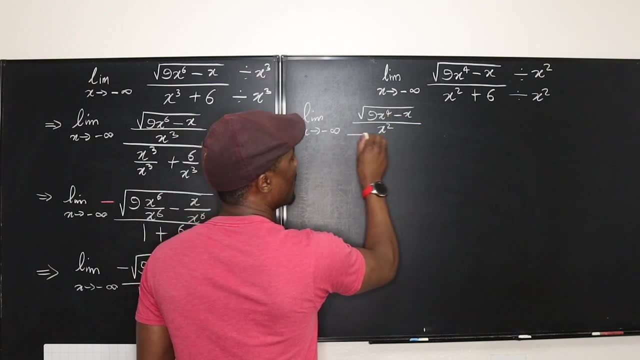 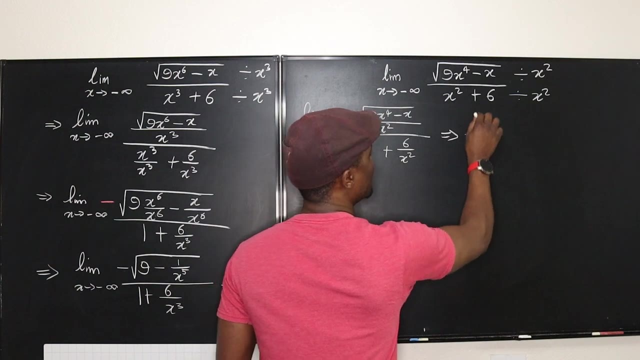 here, which is x squared. Divide this also by x squared, So I'm going to write it as the square root of 9x to the 4th, minus x, divided by x squared all over x squared over x squared, plus 6 over x squared. Well, this will give us the same thing as the limit as x goes to. 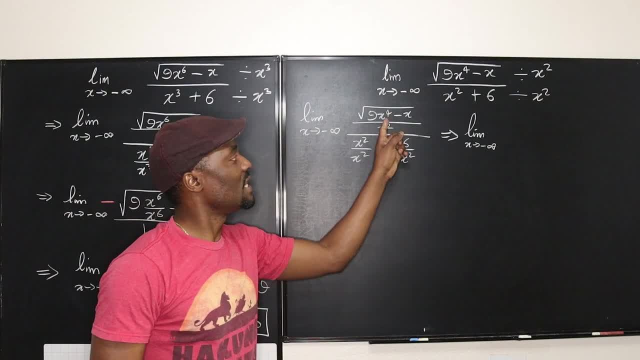 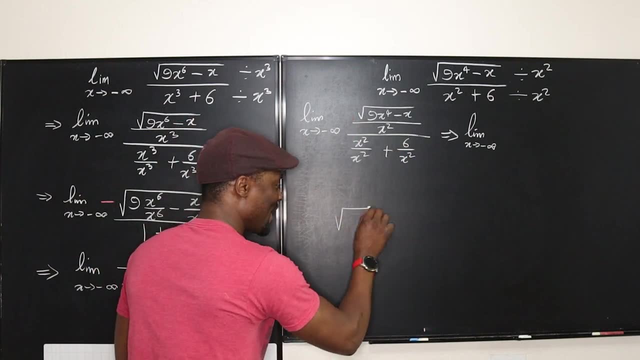 negative infinity of Now, this is going to go in and as this goes in, it becomes x to the 4th. okay, However, we will not need to put the negative sign outside, because the square root of x to the 4th can be written as the square root of x, squared squared, which. 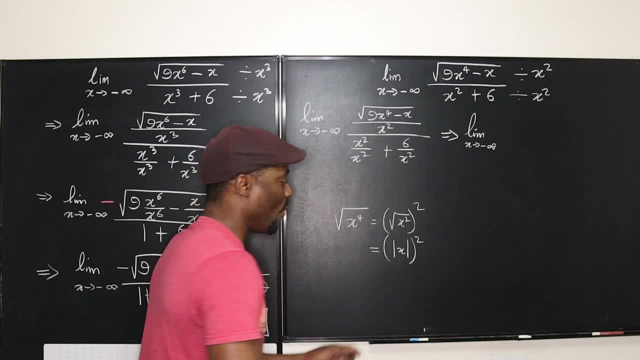 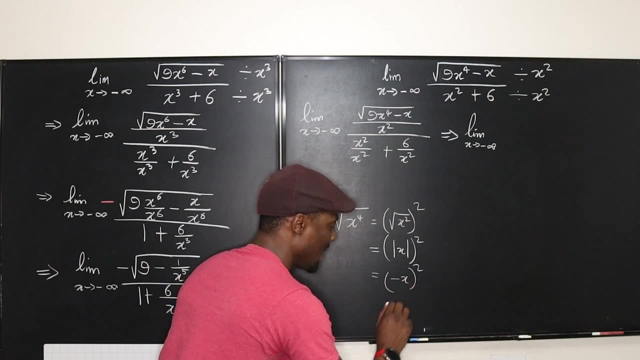 the square root of this will be absolute value of x. and then you square it. Well, what will we choose? We choose the negative, the negative option, because x is approaching negative infinity. So if we put negative x here and then you square it, it will end up becoming just x. 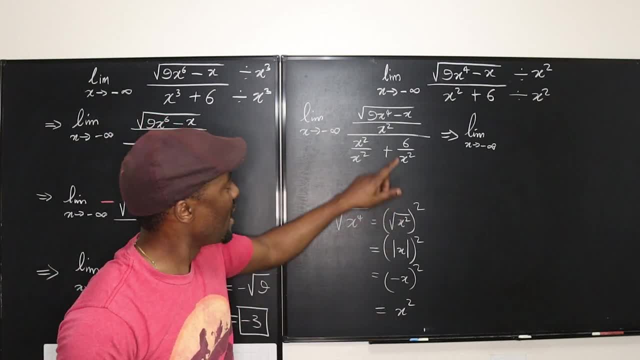 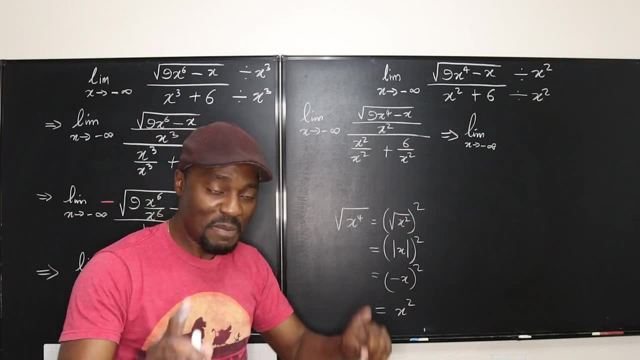 squared, So there's no negative, decided to take outside. It's just going to be x squared, So we'll be dividing x squared by x squared and then that's just it. So that's the reason why we're not taking out the negative sign. You have to remember that. Okay, so I'm going. 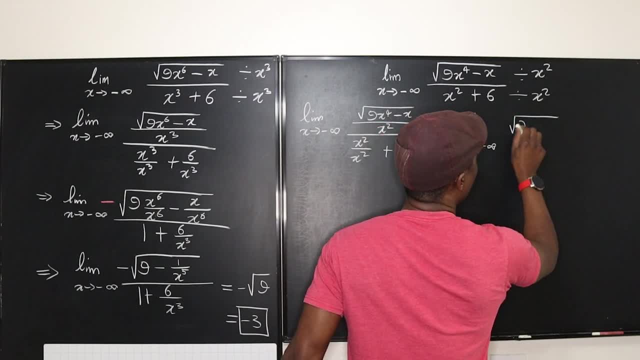 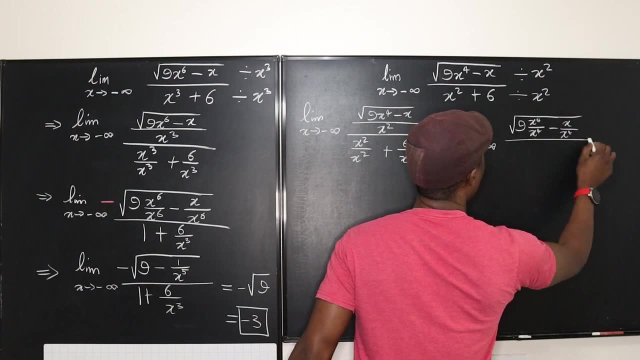 to rewrite this as the square root of 9x to the 4th over x to the 4th, minus x over x to the 4th. Let's write it that way All over. Well, this is going to be 1 plus 6 over x. 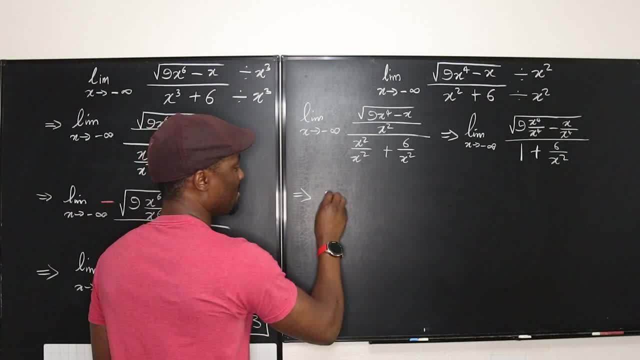 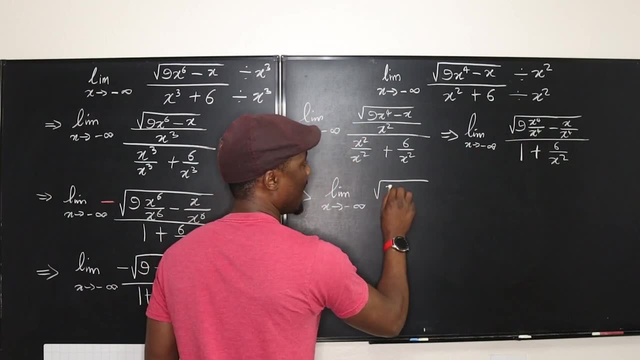 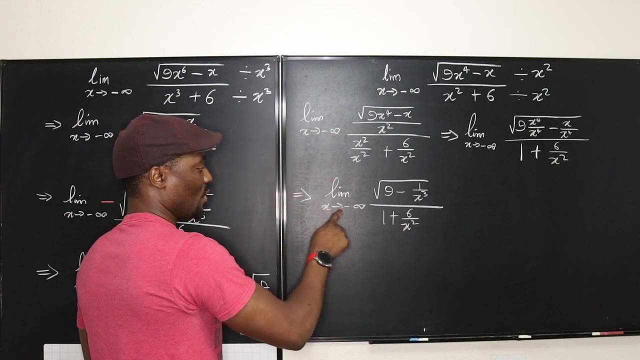 squared. So our next line is going to be the limit as x goes to negative infinity, and if we simplify this, it's going to be the square root of 9 minus 1 over x, cubed over 1 plus 6 over x squared As x goes to negative infinity. this goes to 0, and our next line, 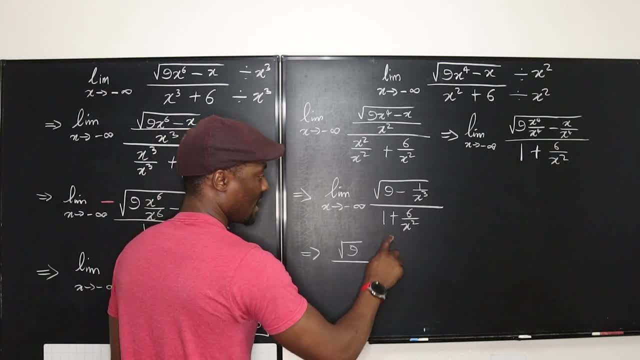 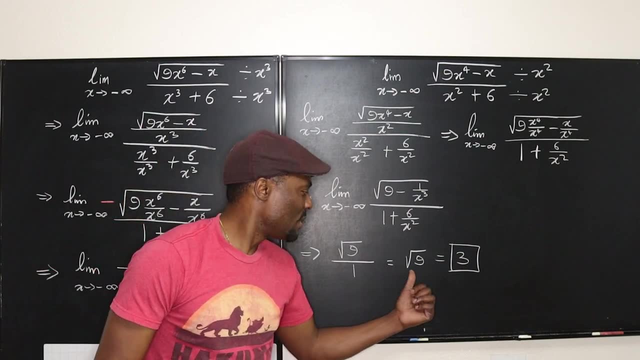 is going to be square root of 9 over. This is going to be over 1,, which is the square root of 9,, which is equal to 3.. Okay, Okay, Now I have a question: When we take the square root of 9,, is it not possible that it's negative? 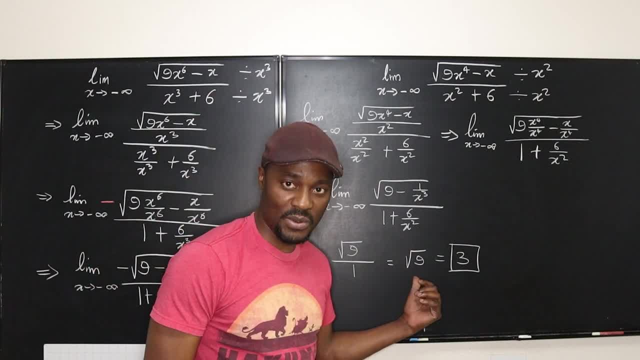 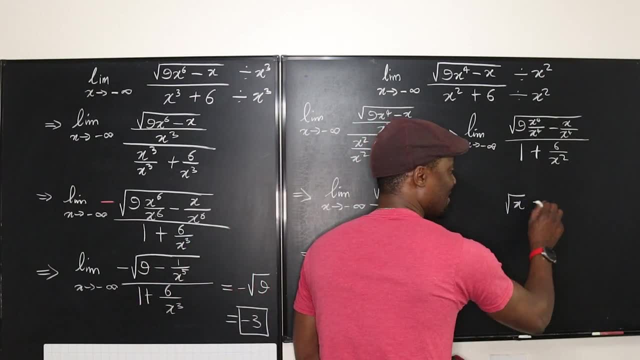 3 or positive 3?? Now remember, when you take the square root of a number, you choose the principal root. The principal root is always the positive root. Remember that. Also, the square root of x must be the positive option. Forget about the negative The only time you. 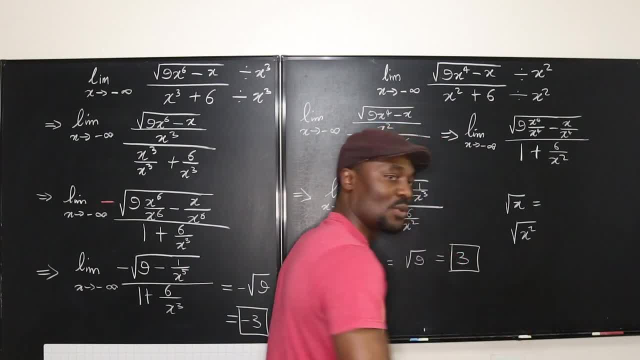 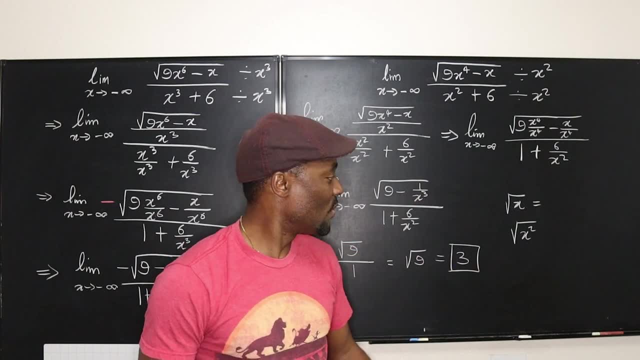 take. the option of the negative is when you take the square root of x squared Now. that's when you start talking about absolute value. In this case, no absolute value. So the square root you take of 9 is the positive option. There's no negative option. 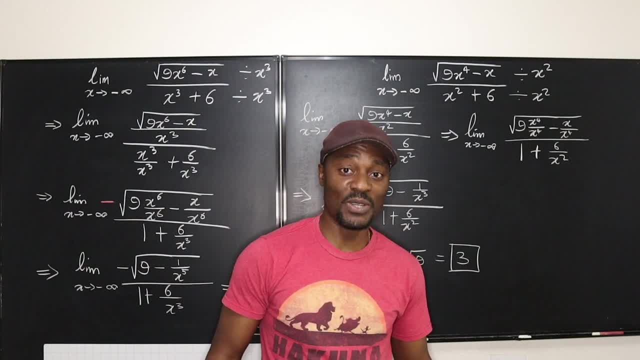 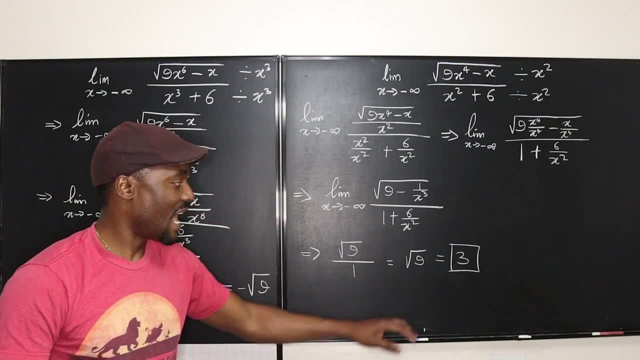 You take the square root of any number, Forget about theed actual number. I hope that works out for you. So that's the whole thing about the difference between this answer and this answer. This answer will be positive, This one is negative. So if you notice that when this is 2 times, 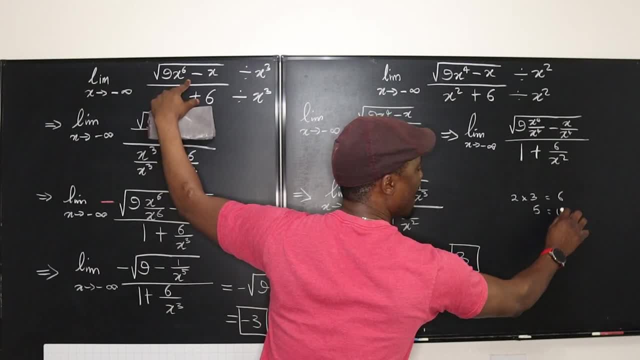 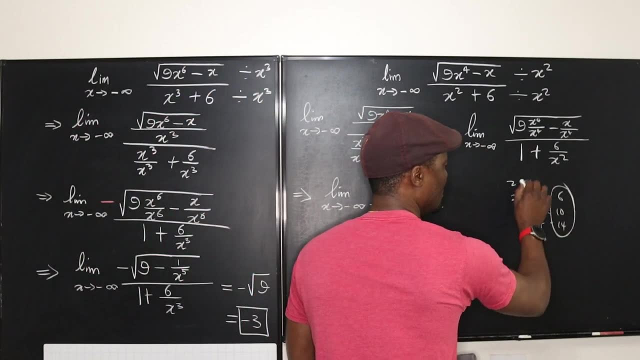 3 and gets 6.. If you all change this to 5, you'll get 10.. If you change this to 7, you get 14.. When the exponent that is here is an odd multiple, the same thing: 1.. 2 x 1.. 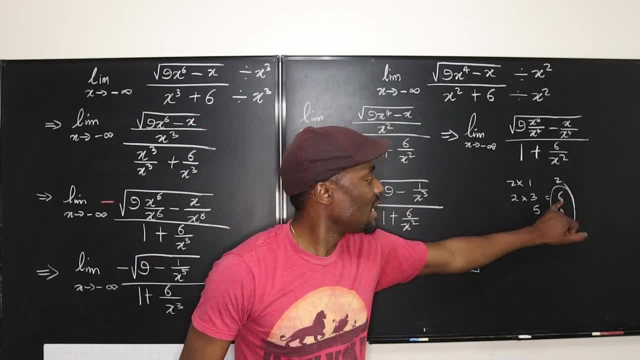 So when you have any questions, just let me know. Thanks for watching. I'll see you in the next video. Bye, where this is under the square root sign: 2, 6, 10, 14 won't be the next number, but 18, once you have. 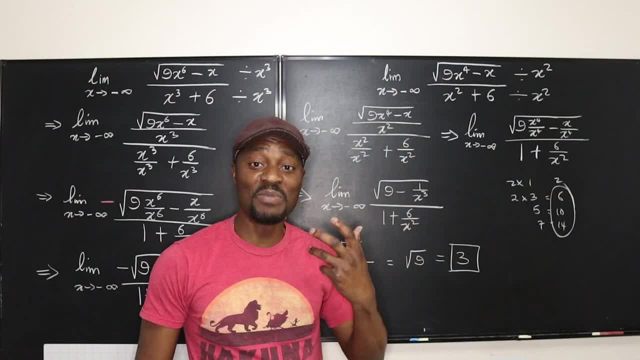 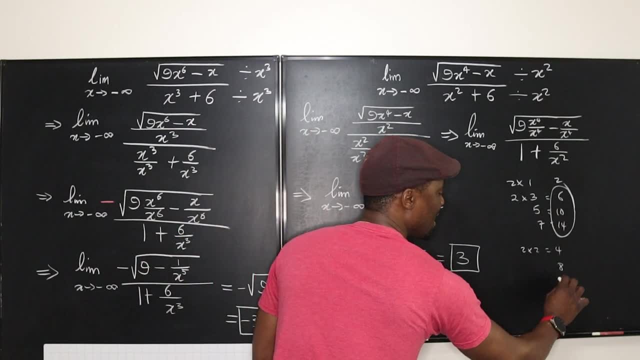 those differences, then you know that your answer is going to be negative, as x goes to negative infinity. but when you have those numbers, such as 2 times 2 gives you 4, and then you have 8 and then you have 12, is it 12? yeah, this is going to be 2. you can have 4, 6, 12 and then all those, even. 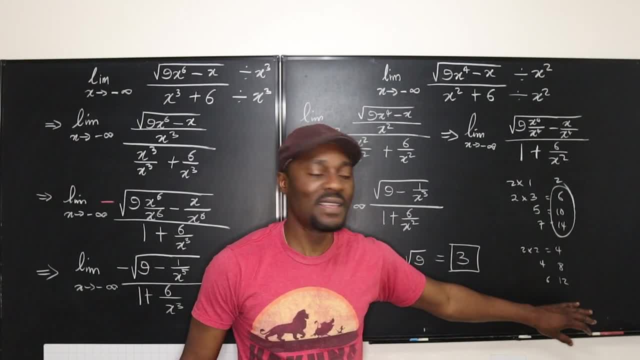 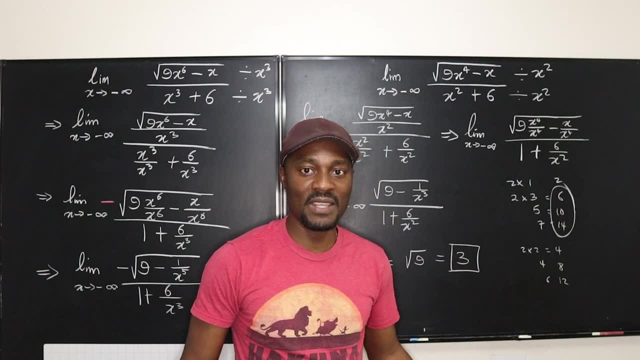 multiples, not even multiples. um, the multiples are 4. okay, i think that's what i should do. multiples, no, not just one, because there's a multiple of 4. just know that when you divide it by 2, you don't get an odd number. then you're fine, it's going to work. but when you divide by, 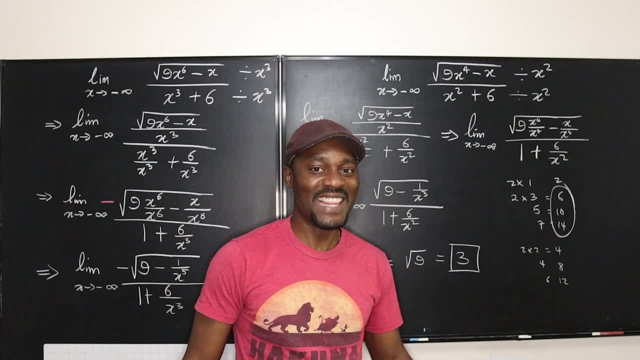 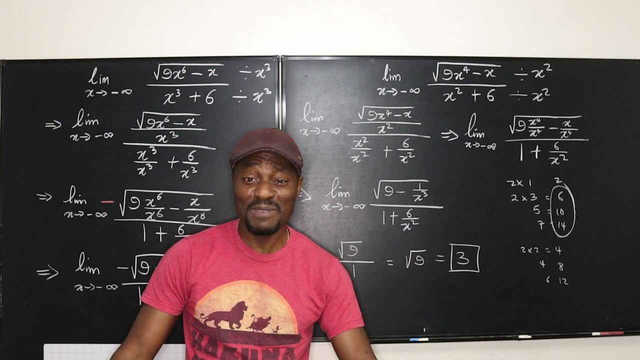 2 and you get an odd number, that's going to be a problem. okay, that's when you must stick to the negative. i hope this video made a difference. if it did, give it a thumbs up, make sure you share it, make sure you like it, leave a comment in the comment section. i'll see you in the next video. 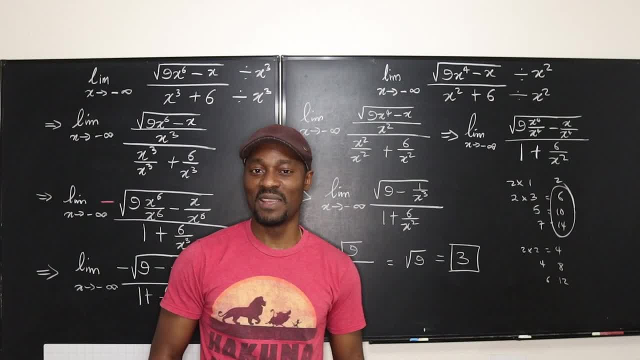 until then, don't stop learning, because those who stop learning have stopped living bye.